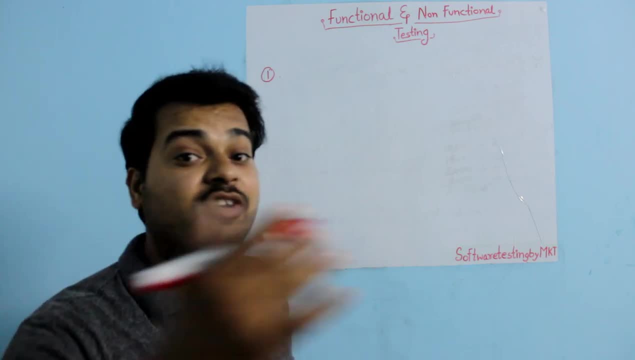 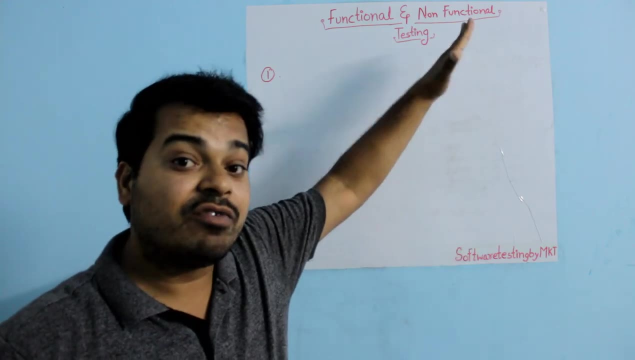 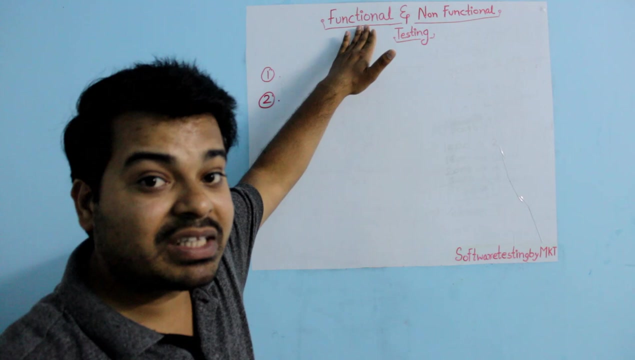 focuses on the performance of your software, the load your software can take, how reliable is the software, how the scalability of your software. so non-functional testing focuses on that. coming to the second point, your functional testing, it is given by the customer. it is a customer who will tell. 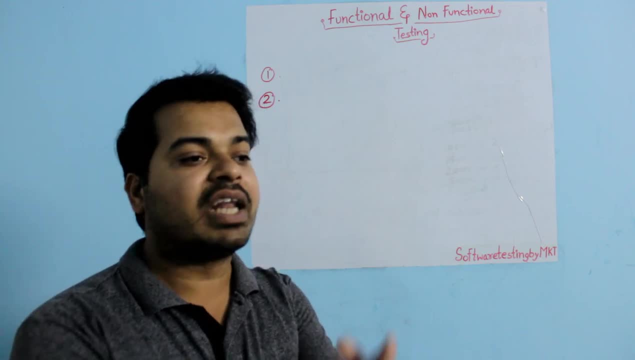 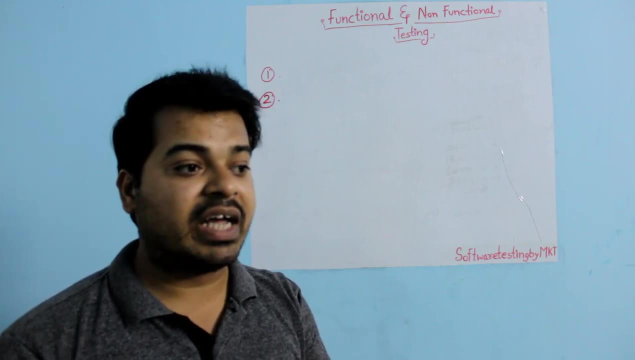 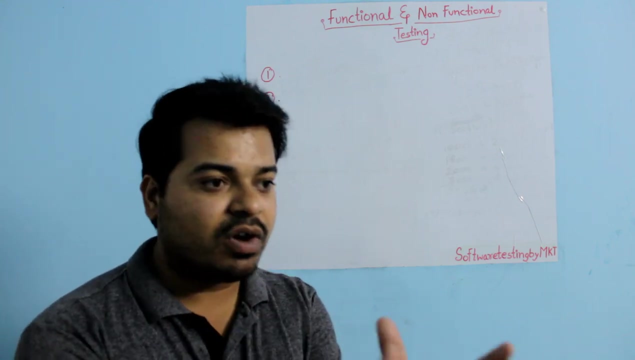 that we want a software which should work like this. it is your customer who will tell the functional requirement they will give that your software should work like this, that we are expecting our software, which you guys are making, should work in this way. so we do functional testing based on the. customer's requirement but we do non-functional testing because of the customer expectation. guys, whenever any company is developing any software for their clients or for anyone, definitely clients will mainly focuses on functional requirement. they give least priority for non-functional requirement or non-functional testing. so customer will give the functional requirement. 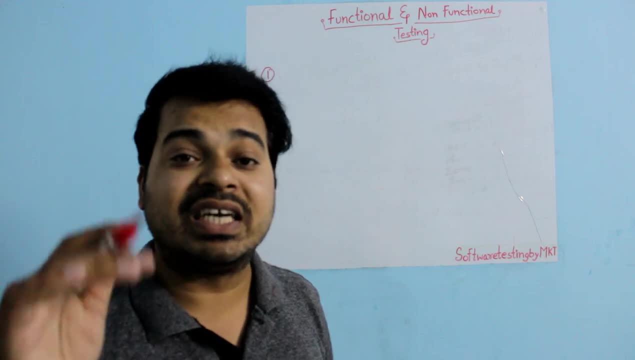 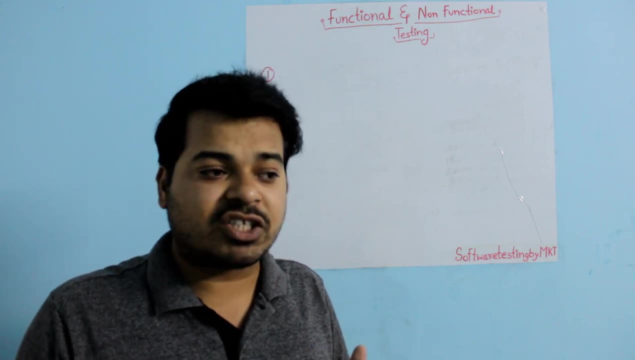 which we will tell you about in the next video. Thank you for watching this video. See you in the next video. Bye, Bye, test it and give it to them. but, guys, it is a duty of your company or it is a duty of your tester or developer that we have to give the software to our clients. 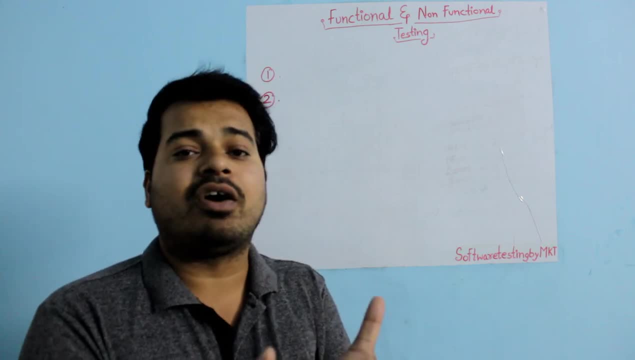 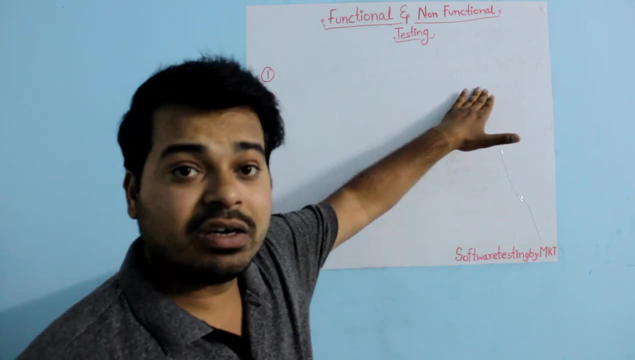 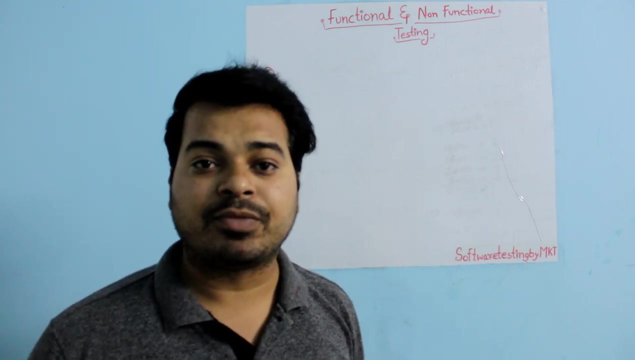 in such a way that they will not come up with the defect or anything in the future or complain. what kind of defect you can expect if you don't do your non-function testing? you can expect that they will tell that the web pages are loading in 50 seconds, or each and every pages of your. 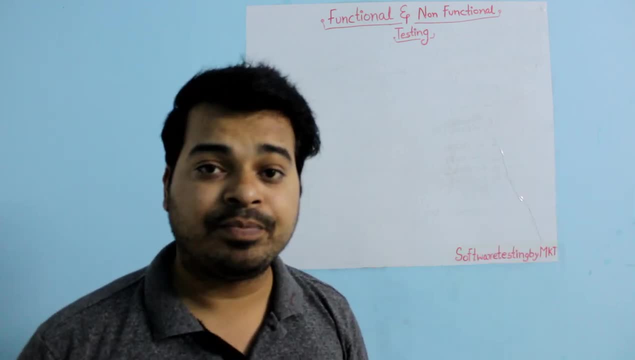 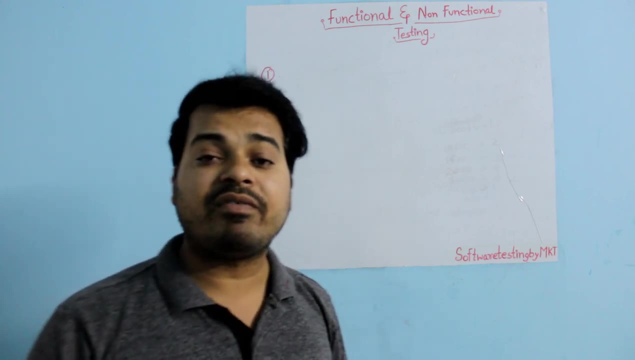 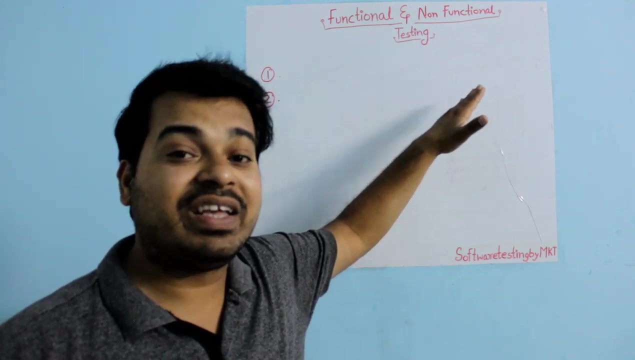 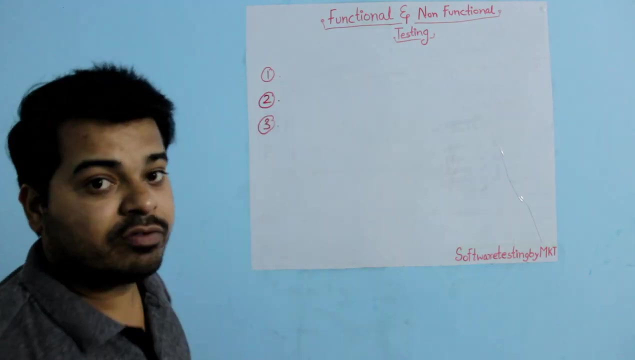 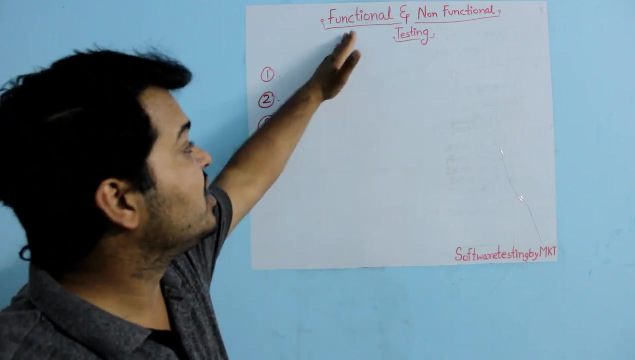 their web pages are taking time to load. they can also tell that there are multiple security defects. so where, as a company, whenever we are developing the software for our customer, we do non-functional testing because we know that customer will have their high expectation from us. now functional testing. so functional testing. whenever we test any software, it is the functional. testing that we test first non-functional testing. we always test once after the functional testing is done. why have you got this question in your mind? so the reason we do non-functional testing later: because till now you would have understood that performance testing comes under non-functional testing. so guys, tell me, when you are developing any software first, you will try to test the. feature in that application, or first you will put load and test whether it is able to handle that load or not. definitely not right. first you will test the feature, which will come under functional testing. later you will do non-functional testing that later you will do your performance testing. 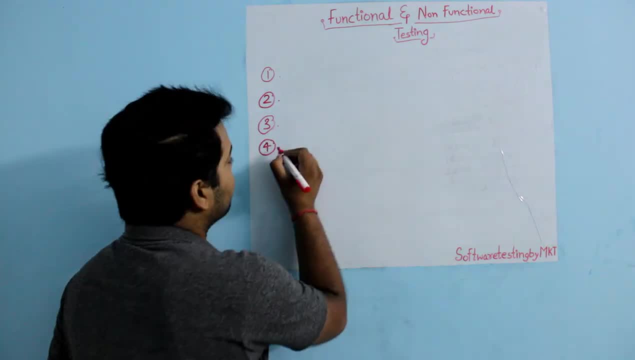 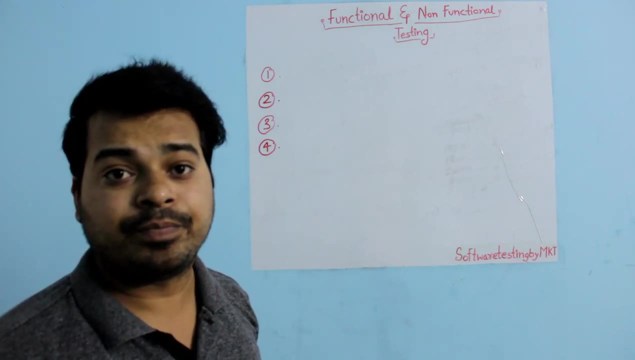 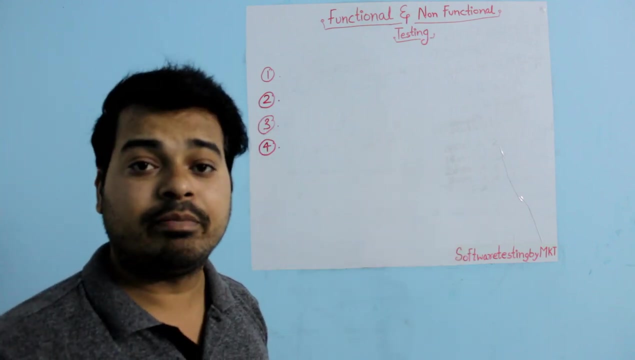 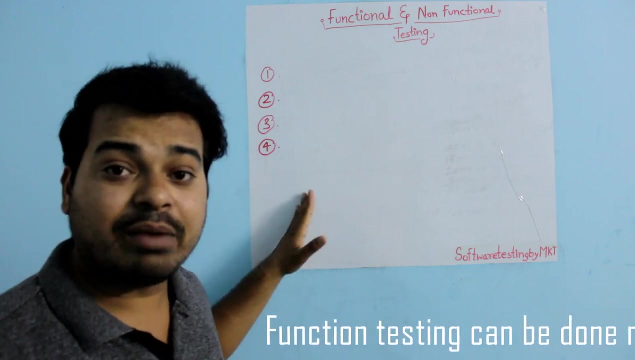 i hope doubts are clear. next, on: all the type of functional testing can be done by manual testing, but all the type of non-functional testing cannot be done by manual testing. it can be done, but it will be a very, very, very, very, very, very tedious process to do. so remember, functional testing can be done by only manual testing. but 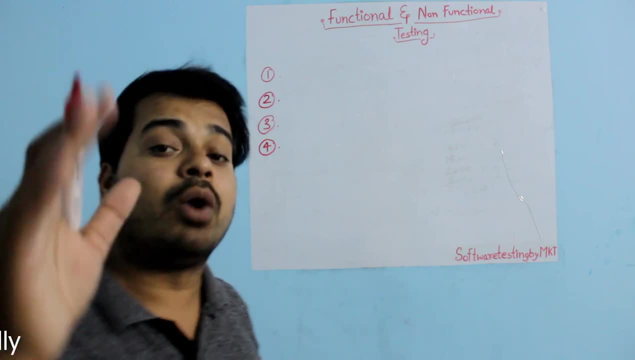 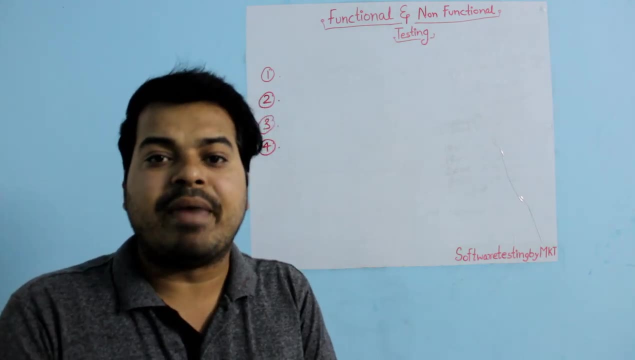 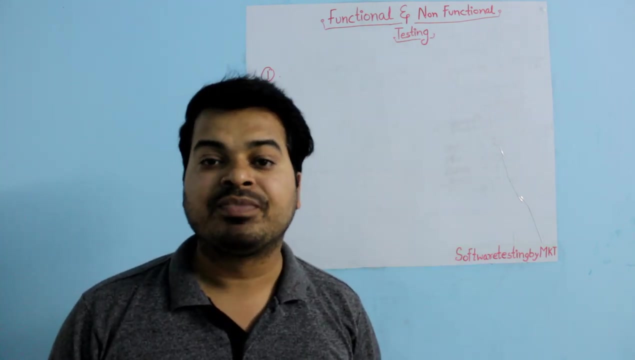 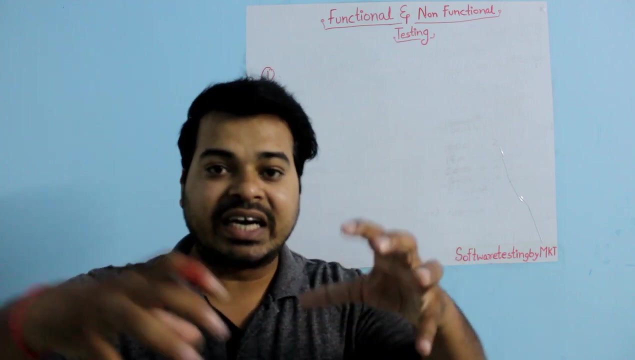 non-functional testing cannot be done by manual testing. how, remember, suppose function, you are testing a feature, you can test it manually. no rocket science here. but talking about your non phone health testing, suppose you are doing your performance testing and you want to check that whether my software is able to handle one lakh of requests at a time. 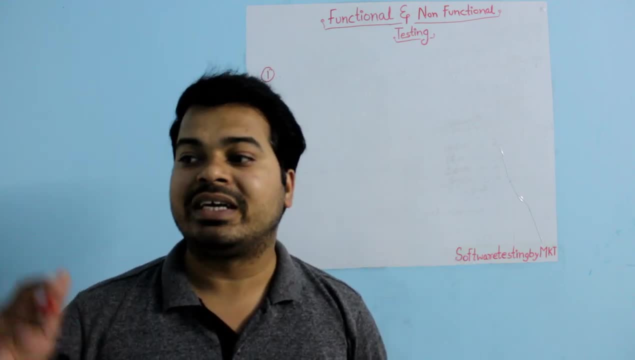 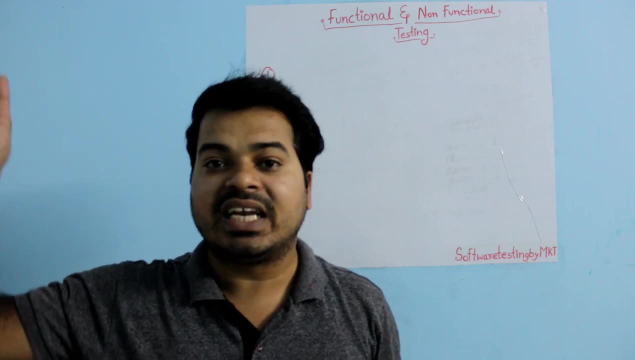 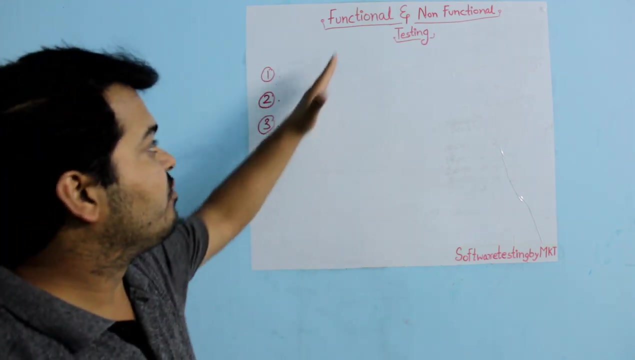 or not, what you will do. is it possible for you to put one lakh of laptops and then send a request at a particular moment of time? will you assign one lakh of testers to test that application? it is a tedious alright. that's why I'm telling man, functional testing is always possible to do manually, but non. 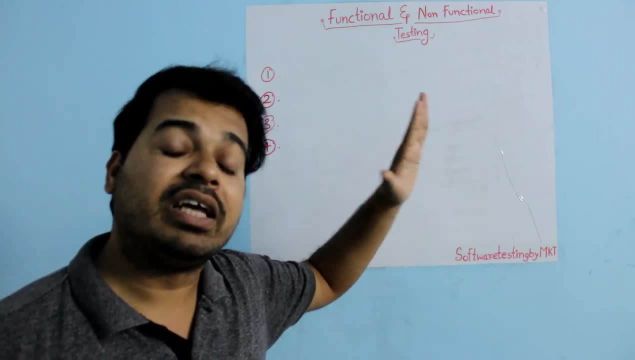 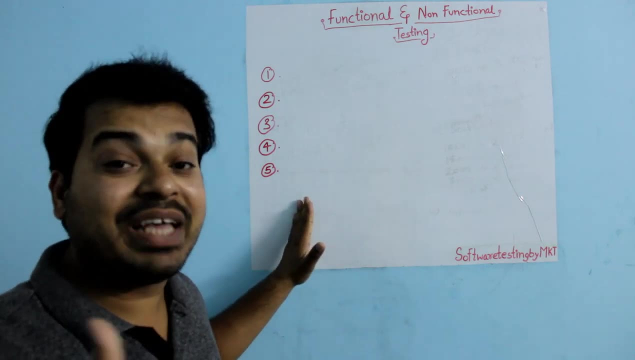 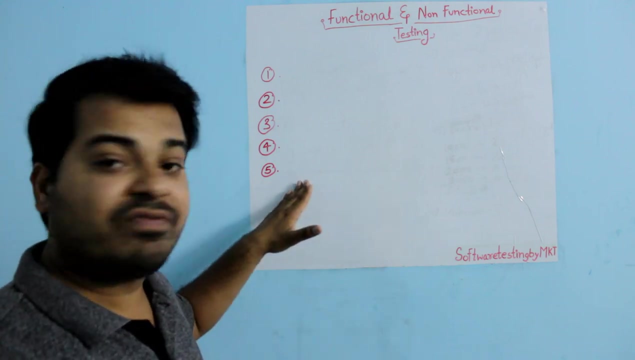 function testing is not possible to do manually. it is, we can do it. it will be a very tedious job. functional testing which at the behavior of the application. in non-function testing, which add the performance of the application, since in functional testing we will test whether the functional 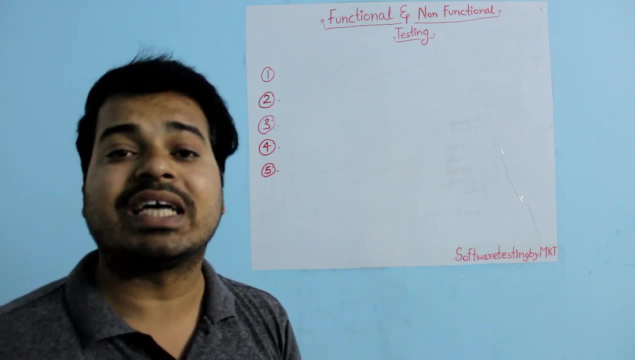 require that we need a number of test already: do faster testing and the speed testing which is one of the interface related to automation under the application. in non function testing we check the performance of the application since, in whatever the customers gave, our software is working as expected or not. in 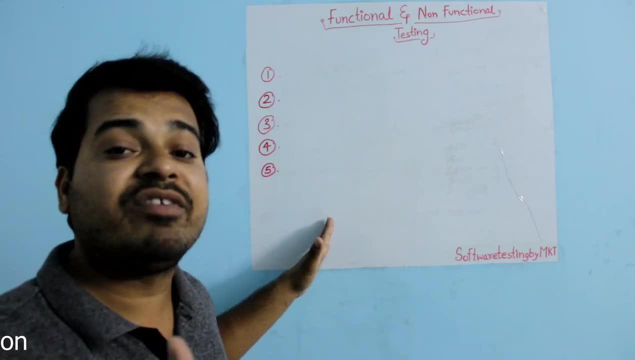 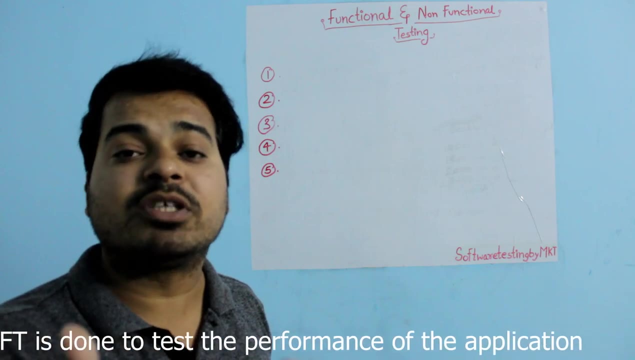 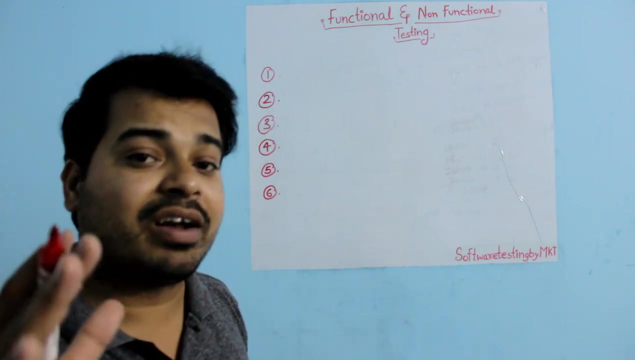 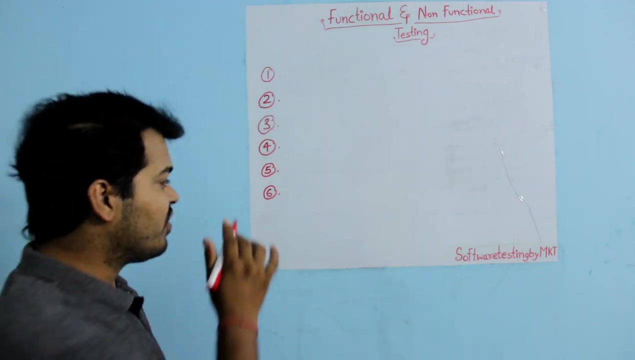 functional testing. we will may focus on the behavior of the application, but when it comes to non-functional testing, we will make sure that whether the performance of the application is good or not. six point: now the question arises: what are the types of functional testing and what are the types of non-functional testing? so the types of functional. 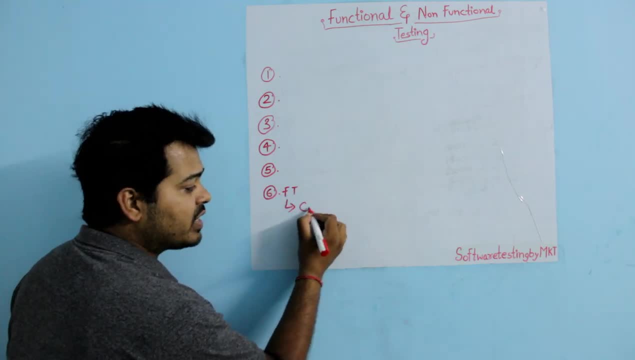 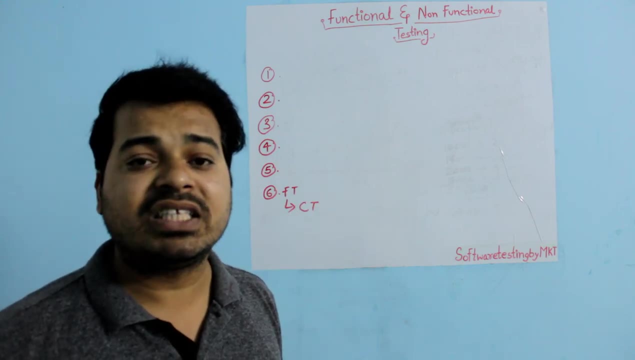 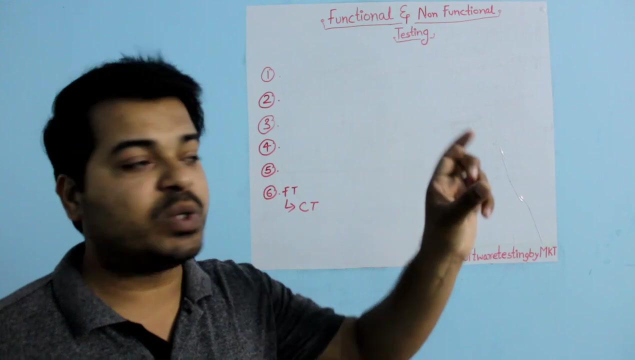 testing we have is your component testing, because in component testing you will test each and every component of the application, that is, if you have any application. let's say, if you have any application in which you have text field like enter your username, enter your password, those components are call. 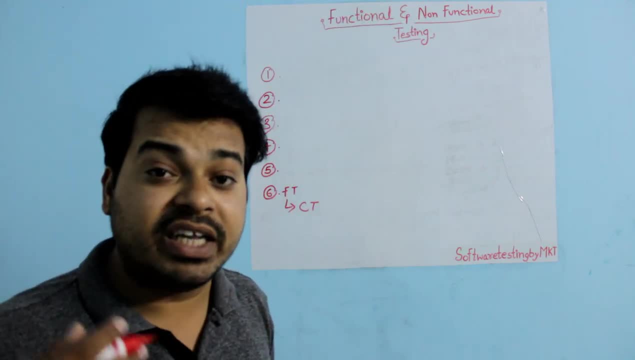 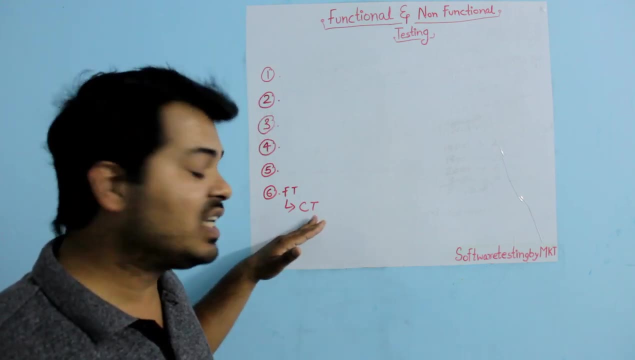 component, if anything which you feel, that is, there is no current challenge, anything that is not correct. so if so, you feel the new to you. i have added all the link in the link description. please go and watch it. all the terms which i'm using: i have already made a video and it is in the link description, if you feel anything. 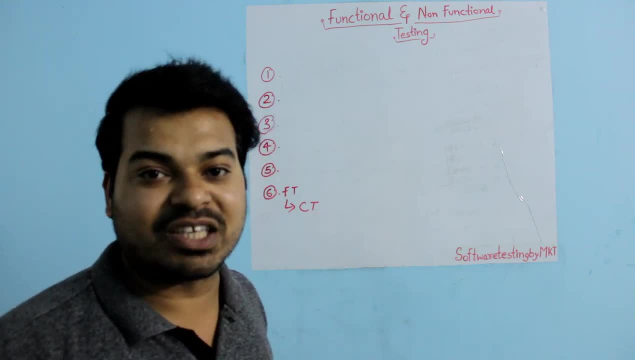 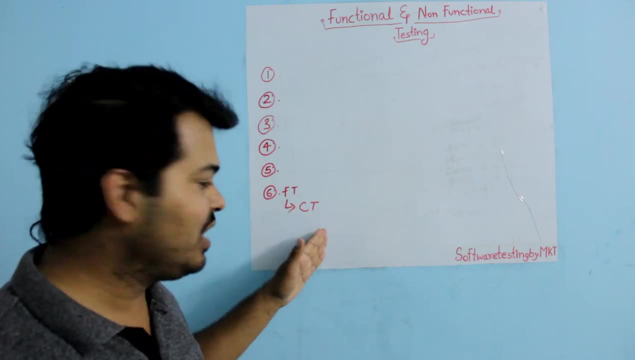 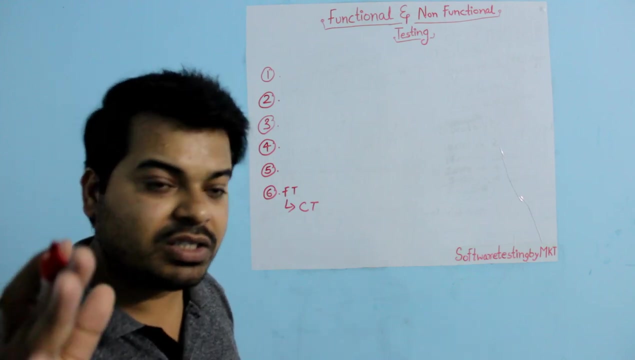 like. if you feel that component testing is not clear to you, it is in the link description. please go watch it and come to this video. so functional testing examples are component testing, because we will test each and every component. why we are testing each and every component? because 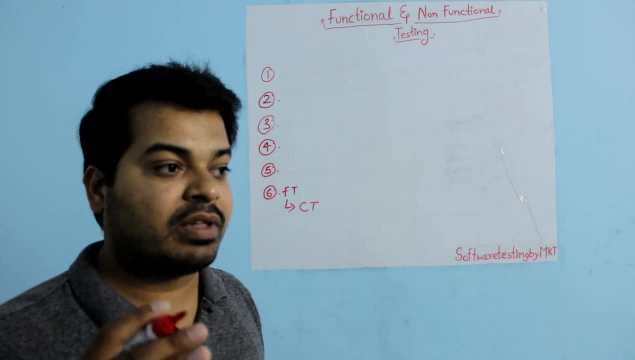 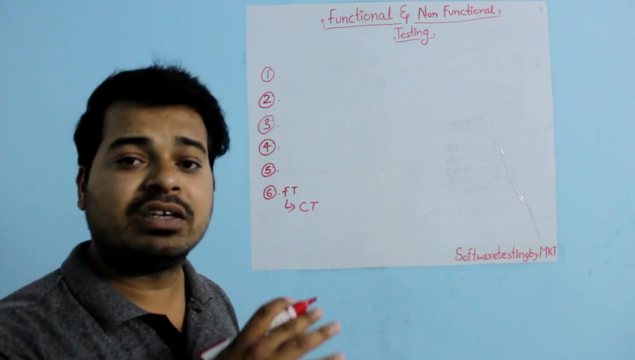 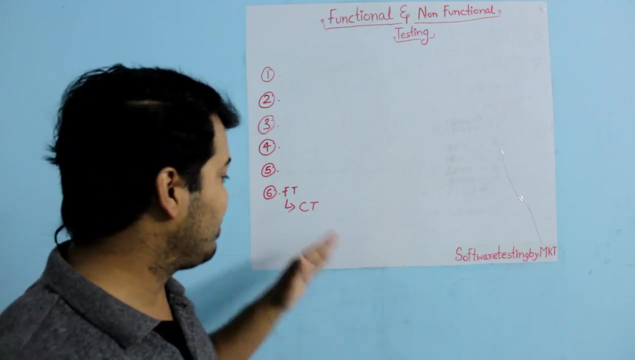 we are doing component testing to make sure that at later stage we have to test if our the integration flows are working perfectly fine or not. we have to test at the system level whether the software- see at the system level- it is working fine or not. so that's why we are doing component. 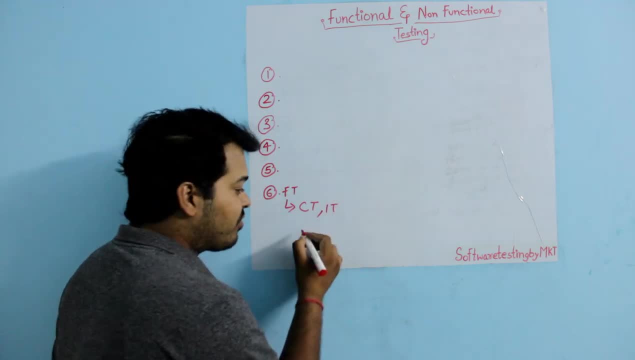 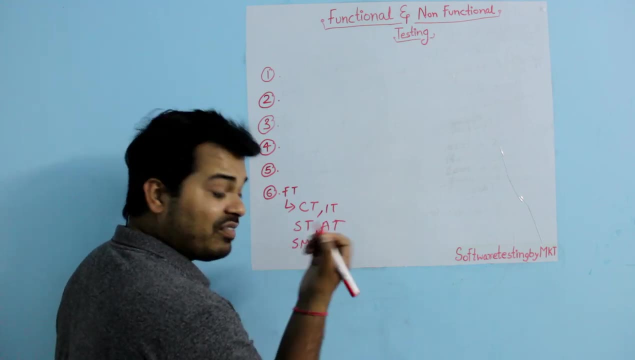 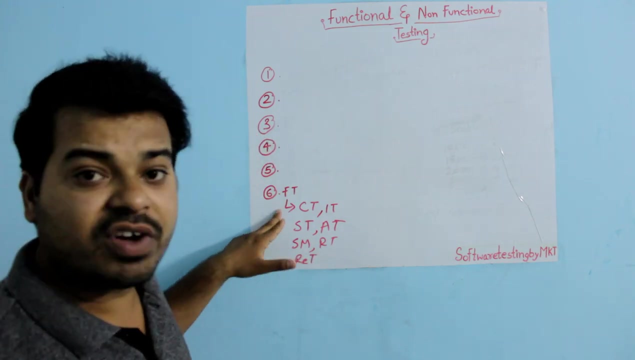 testing. after that we have integration testing. after that we have system testing. after that we have acceptance testing. after that we have smoke testing, we have regression testing, we have re-testing. all those testing comes under your functional testing. each and every video: it is there in the link description. please check it. 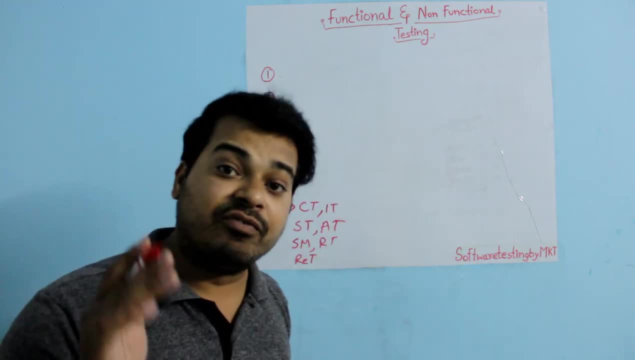 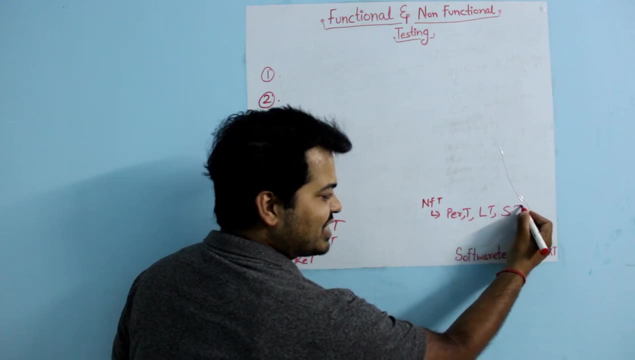 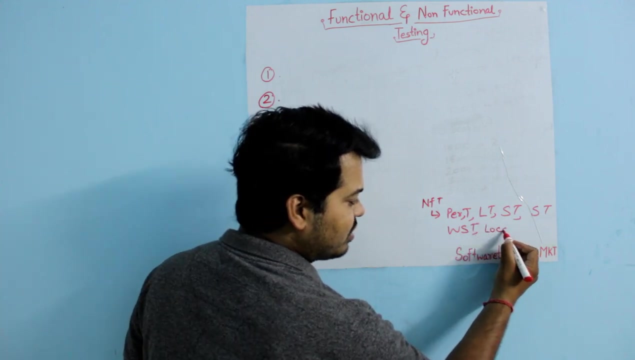 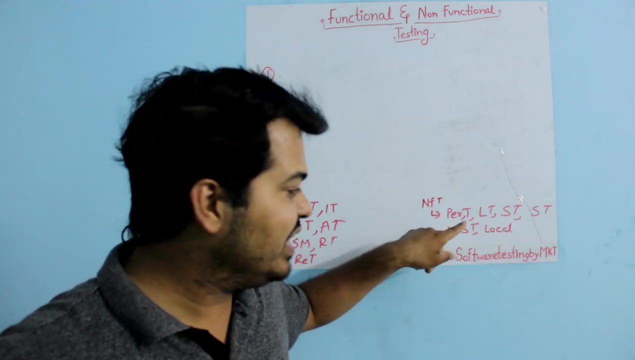 talking about the types of non-functional testing we have. we have examples are: performance testing testing, load testing, stress testing, soak testing, your web security testing, your localization testing- all this will come under your non-functional testing. all these are there in the description for each this type of testing. i have made a video and it is there in the description. 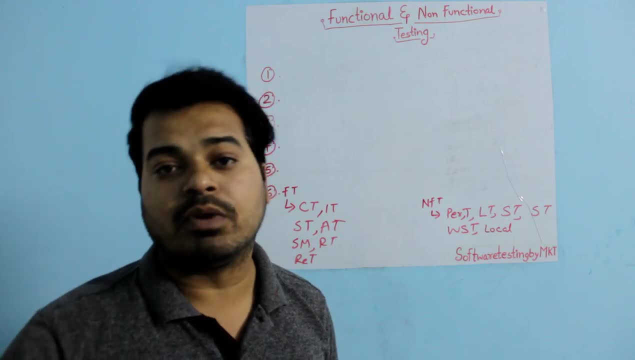 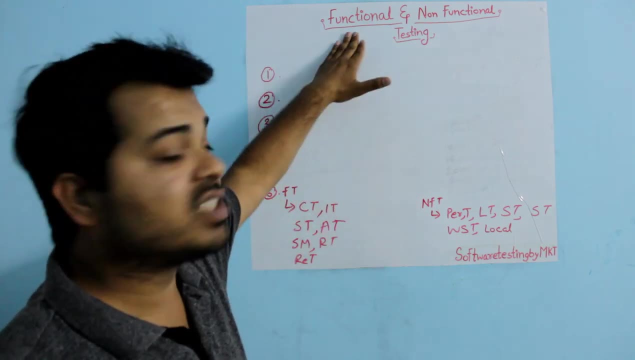 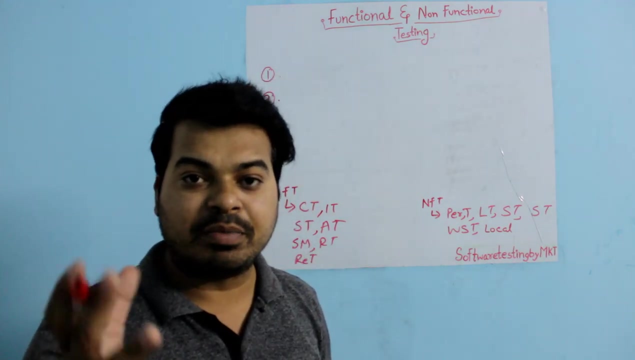 please check it out. before i close this video, let me tell you, guys, one more thing. whenever customers give the requirement they may focus on functional, they mean that functionally, their software should work perfectly. so whenever your developers are developing any software before giving it to the customer, it 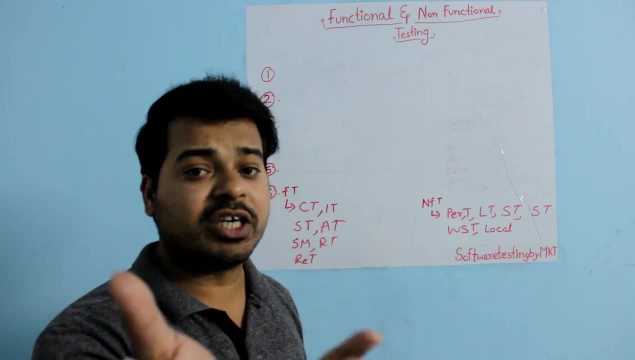 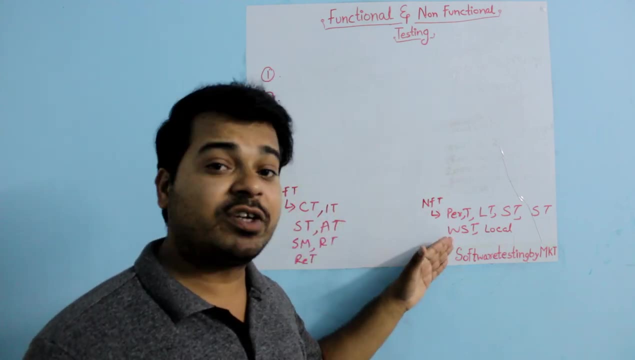 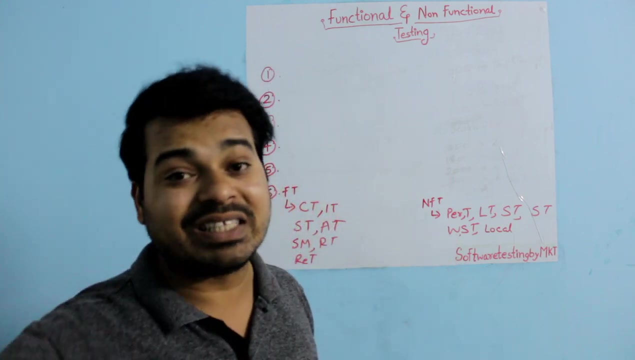 should be your moral duty every testing years. moral duty it should be that you guys do non-functional testing. you guys should keep in mind that your software should not have any web security bugs. now what is web security testing? i have explained in the video. it is there in the link description. please check it out. it is your duty to do web security testing.